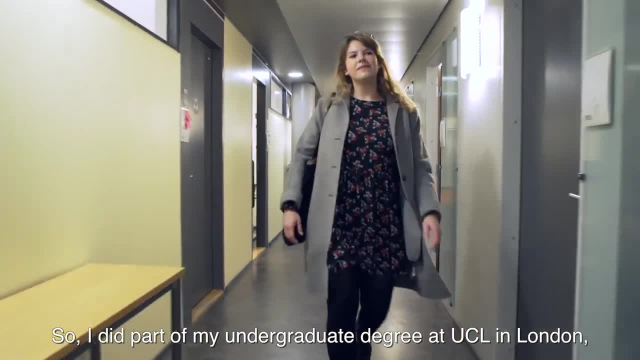 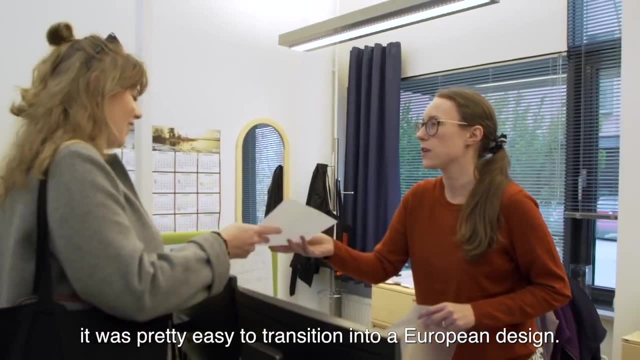 So I did part of my undergraduate degree actually At UCL in London. So already being in Europe, it was pretty easy to kind of transition into kind of a European design. So there's a process. You had to go and apply for it at the embassy or things like that. 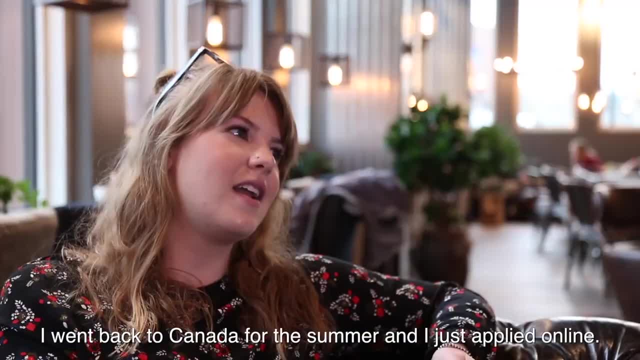 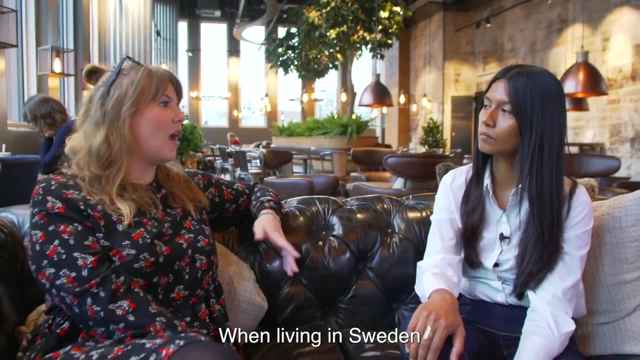 Yeah, So for our visa. I went back to Canada for the summer and I just applied online. The Swedish visa was pretty easy. that factor, And then also when living in Sweden and knowing that I was going to eventually move to Finland. 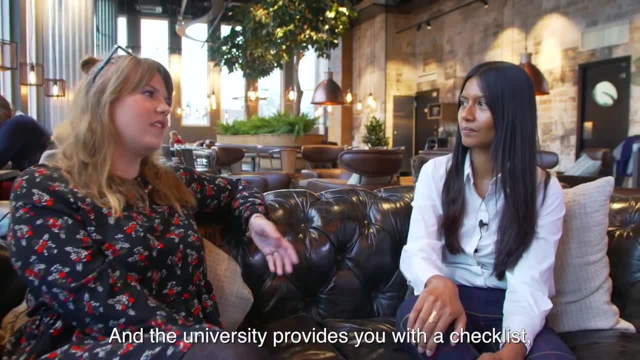 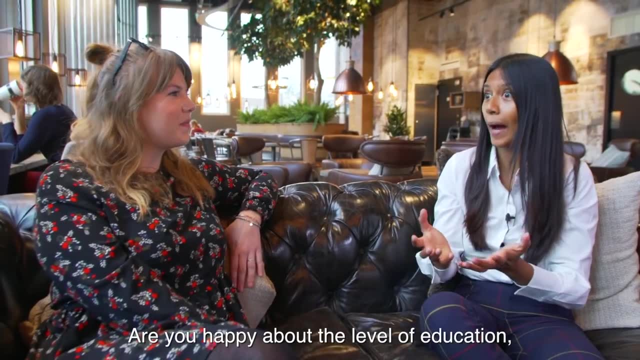 I just went to the embassy and filled everything out. It was a really easy procedure And the university provides you with a checklist so you know exactly what to do to ensure that you are fine when you do get here. And what about the standards? Are you happy about you know the level of education, the teachers? 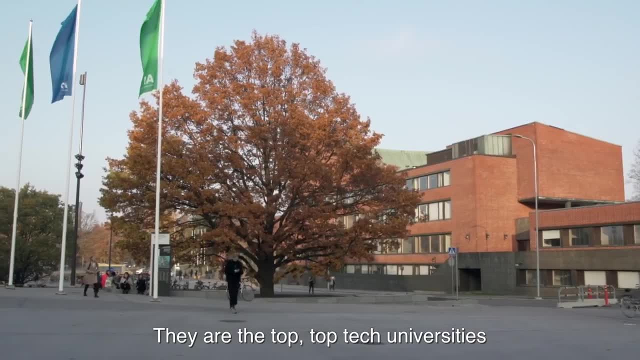 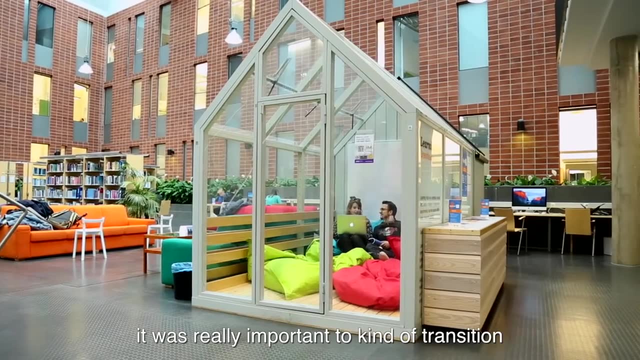 So that was another thing within EIT. I mean, they are the top, top tech universities within Europe. So of course meeting that standard for my undergraduate was really important to kind of transition it through my professional studies And how is life on the campus? 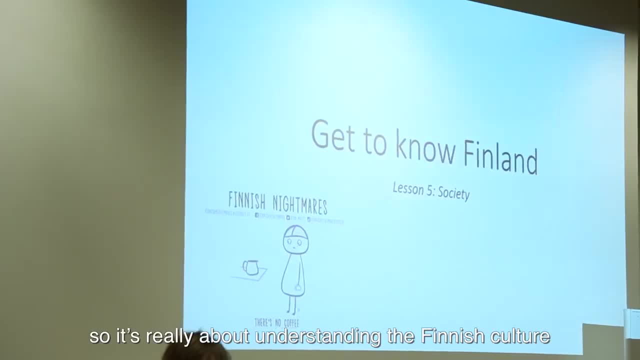 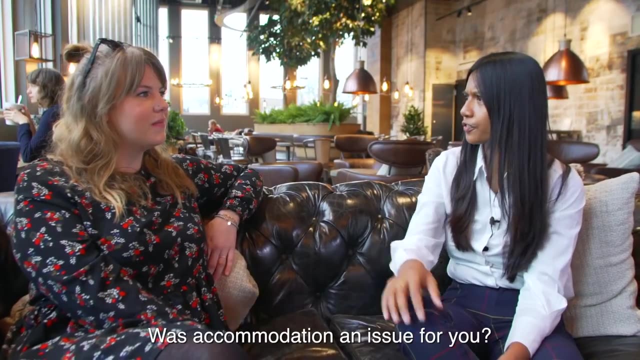 For me personally. I take a Get to Know Finland course here, So it's really about understanding the Finnish culture And how to integrate into society, but also how to compare it to your own. Was accommodation an issue for you In Sweden? it wasn't, because we were guaranteed housing, which is really nice being in Stockholm. 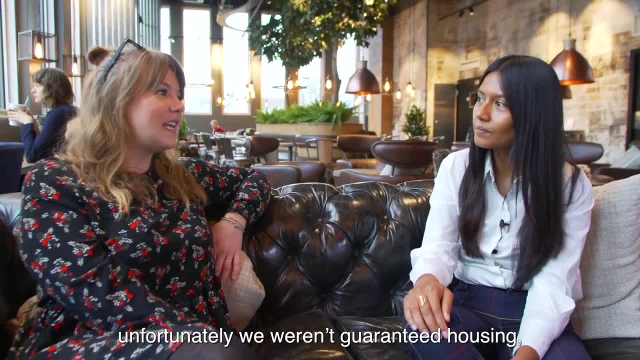 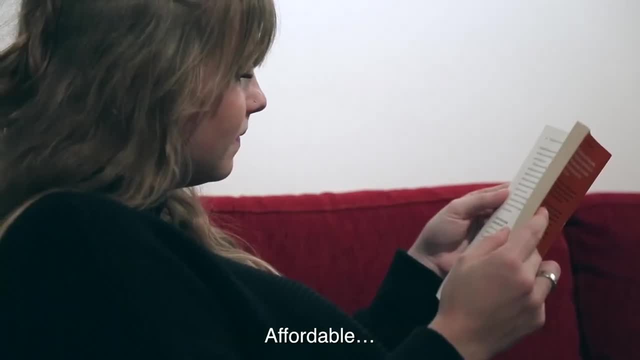 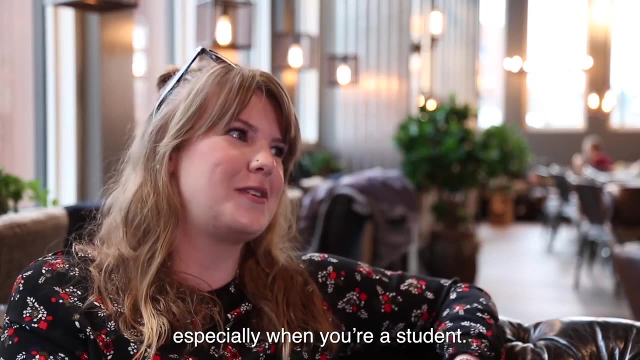 And now moving to another capital. unfortunately we weren't guaranteed housing, But there are tons of programs that you can like sign up for and really help you figure out what Affordable. Yeah, yeah, Also because living in capital countries, obviously that's a main cost concern, especially when you're a student. 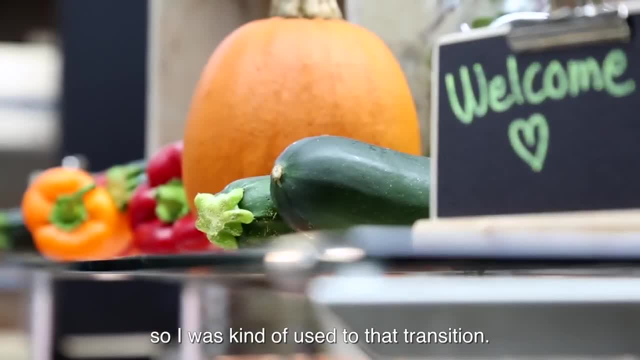 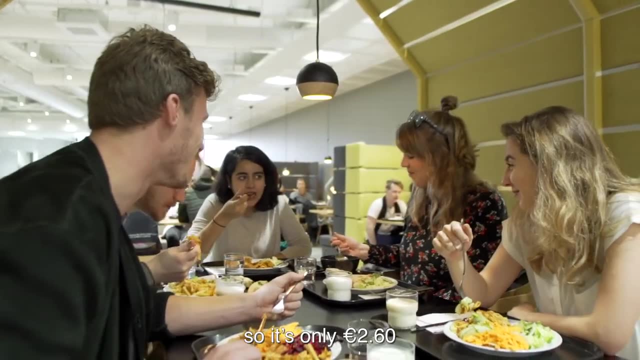 What do you eat here? Finland has pretty similar food to Sweden, so I was kind of used to that transition. We also here have canteens that are subsidized by the government. So it's only €2.60,, which is pretty good. 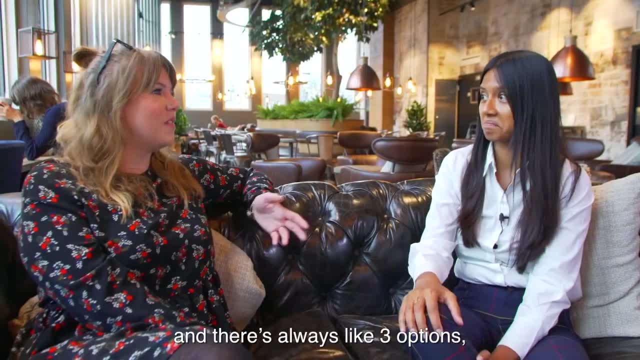 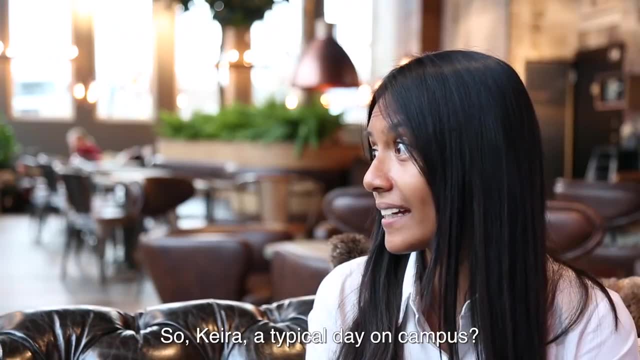 And we usually all have lunch together And international food. Yeah, yeah, So, and there's always like free options, vegan options, vegetarian, So anything you need, it's always there. Fantastic. So, Kira, a typical day on campus.